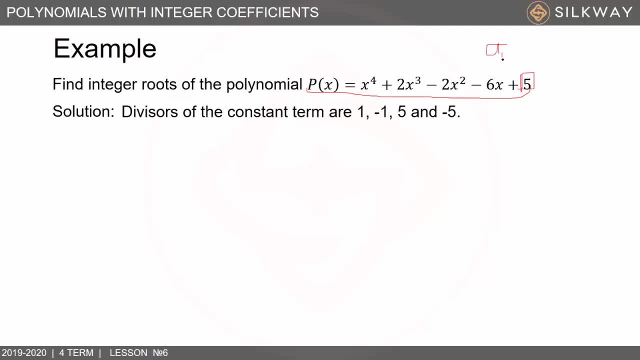 Five. Five is our an is And divisors of the constant term are one minus one. five and minus five. Yes, five has four divisors. Okay, let us find the value of polynomial. at these points. We put these numbers to this polynomial. yes. 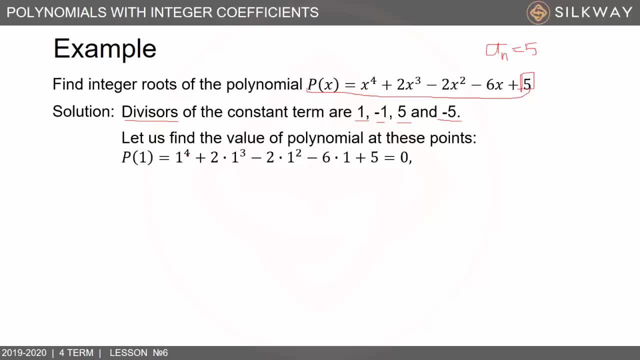 Look, if we put one here, will be one to the four power plus two, multiplying by one cube minus two, multiplying by one square minus six, multiplying by one plus five, equal to: if you solve this expression, you will have zero. 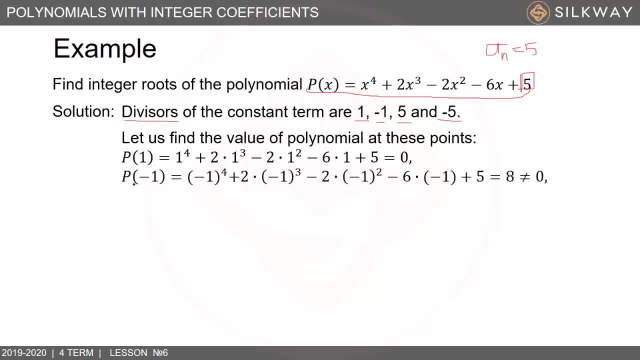 Okay, next one: If we put minus one, here will be eight. Eight is not equal to zero. And let us put five, Here will be eight hundred, And it also is not equal to zero. And the last one: if we put minus one. 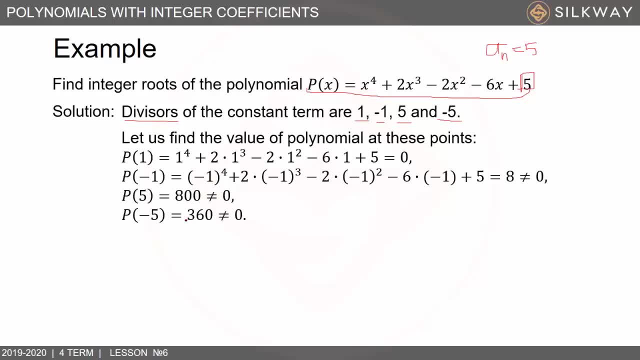 five to this polynomial, we will have three hundred sixty. From this expression we can say one is the root of polynomial, whereas minus one, five and minus five are not. And we can factor polynomial in the form: p of x is equal to. 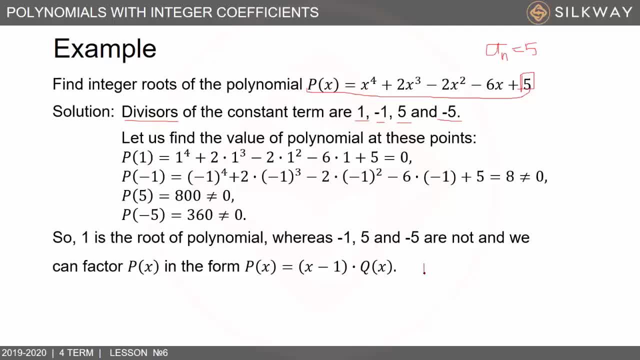 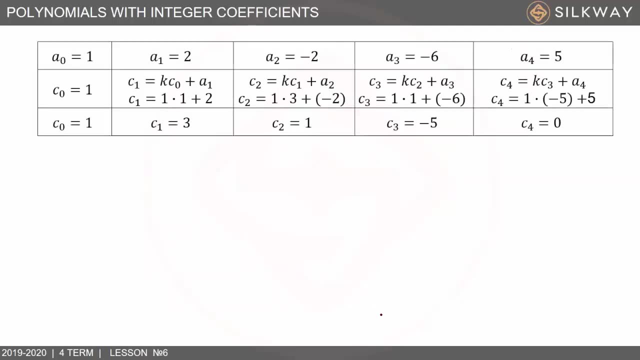 x minus one multiplying by q of x, Here our k is equal to one. Okay, Let us factorize polynomial p of x using synthetic division. We draw a table, yes, and write in the first column coefficients of our polynomial and in the second column 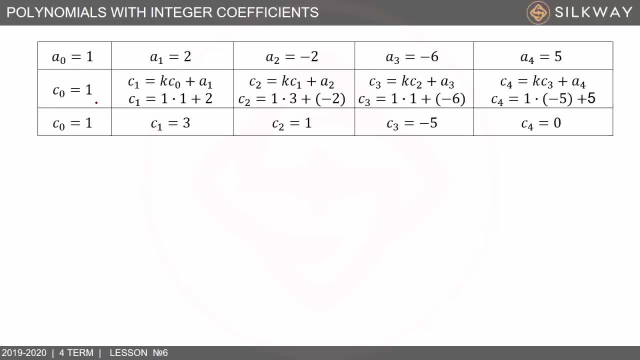 we just find coefficients of our q of x. Okay, We know that a0 is equal to one and c0 also will be equal to one. And then by this formula we just solve, we just find c1.. c1 is equal to three. 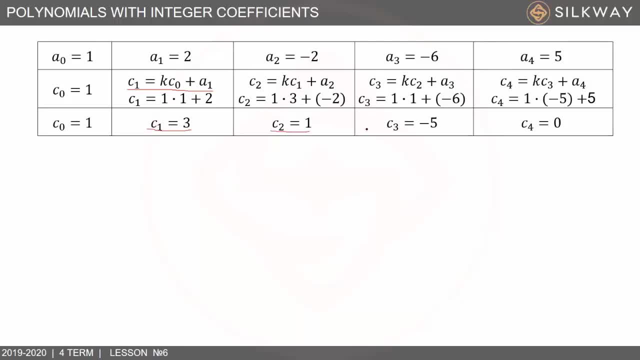 and like that we find our coefficients of q of x, And then we can write like this: Our polynomial is equal to this one is q of x. Yes, And this one is our factor. If we multiply these two expressions, we will have our polynomial. 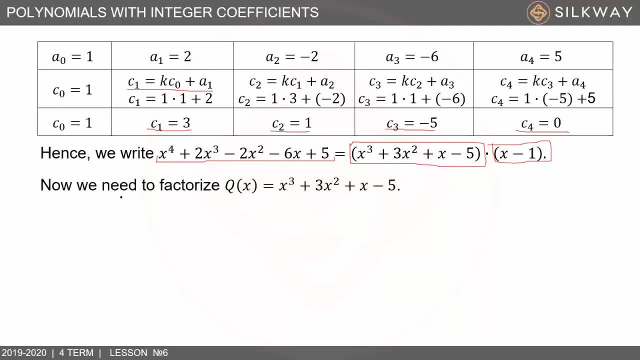 And okay, Now we need to factorize q of x. Divisors of constant term are one minus one, five and minus five. Here is our constant term: yes minus five, And the divisors are these numbers. There is no need to check. 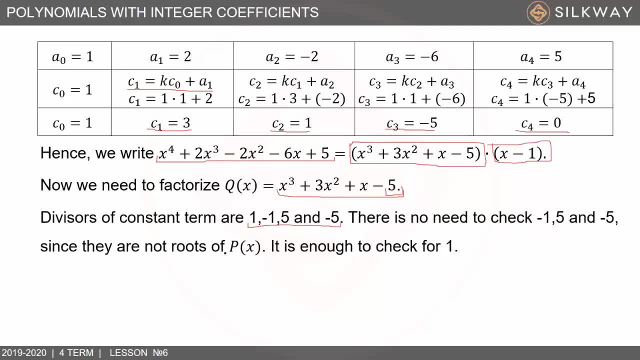 minus one five and minus five. since they are not roots of our polynomial, It is enough to check for one. Okay, q of one is equal to one q. we just put to this x one, yes, and it will be our root. 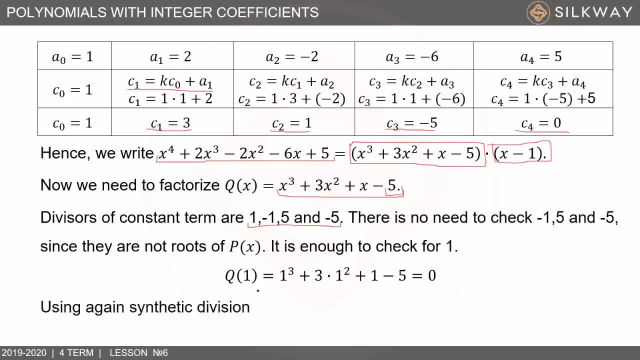 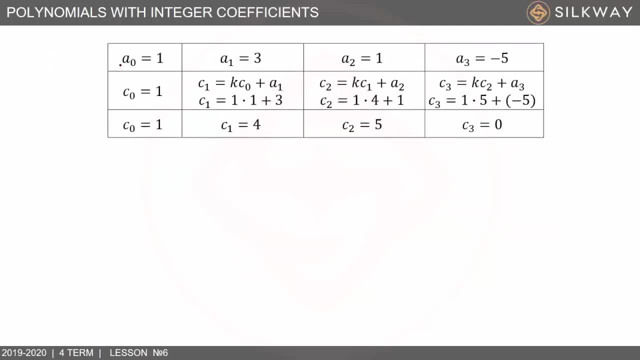 Using again synthetic division. we draw a table here and write our coefficients of q, of x. yes, minus one, five and minus five, And we are solving this. one Here will be: c one is equal to four, c two is equal to five. 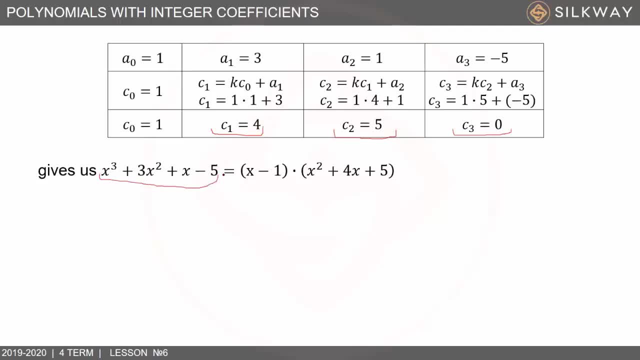 and c three is equal to zero. And then it gives us this expression: is equal to x minus one multiplied by x square plus four. x plus five. This one we get from this table, So we can write x minus one multiplied by x square plus four. 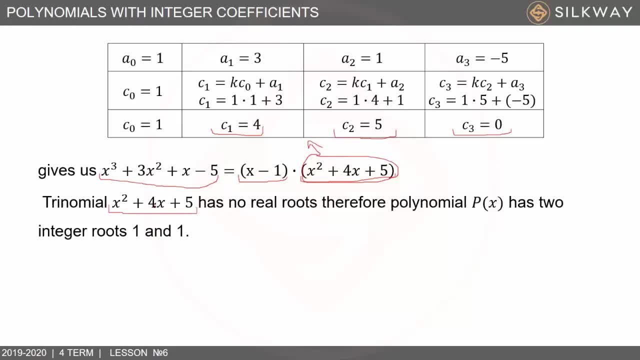 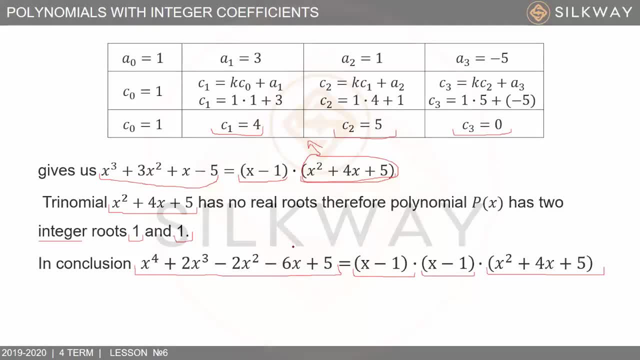 and they are one and one. I think you understand this information. See you on the next video. Good bye.